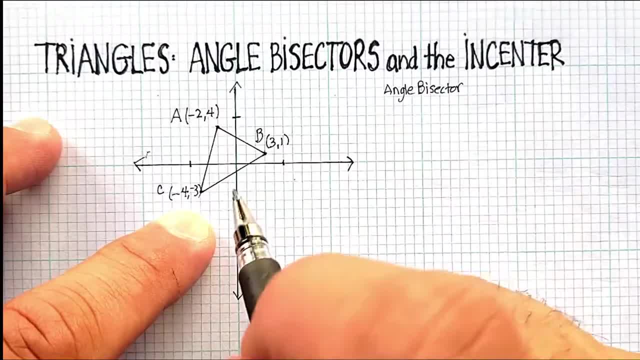 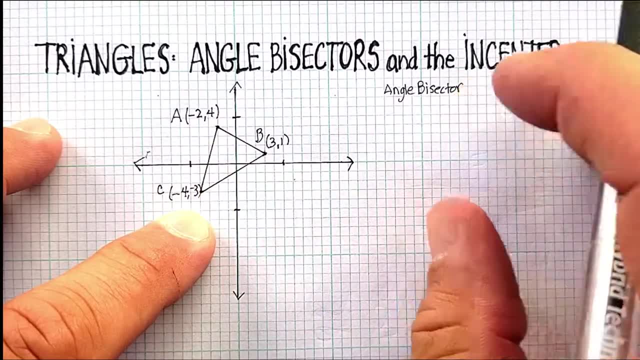 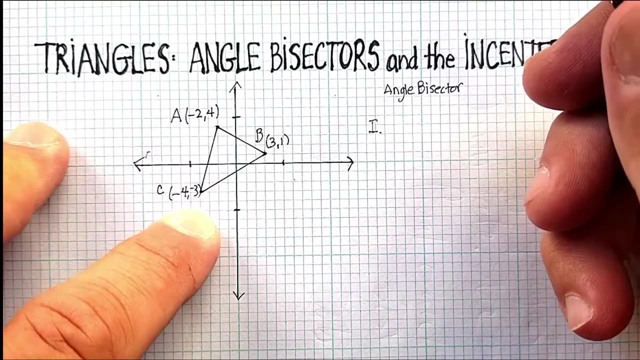 side. okay. So in order to do that, that, we need to find what the midpoint is of each of the sides of the triangle. So one of the first things we're going to do is find- We'll call this our first paragraph in this long journey to figure out what the incenter is. 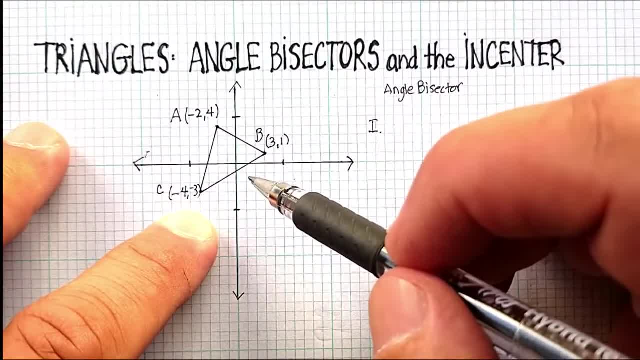 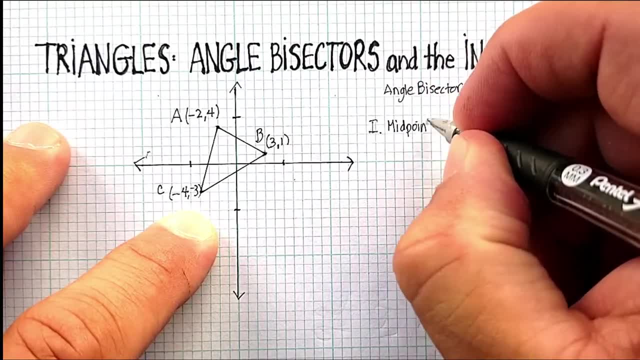 By the way, the incenter is where all those ō lines actually meet, okay, So first things. first, let's find the midpoints of each of the sides of this triangle And notice, I put A, B and C here as well. So let's start with. 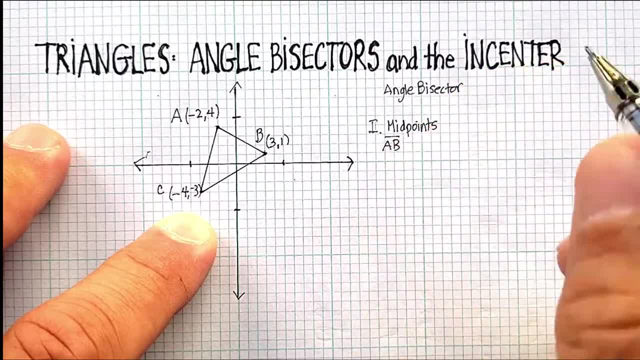 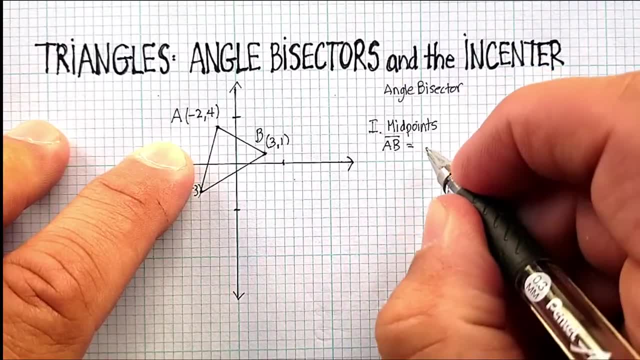 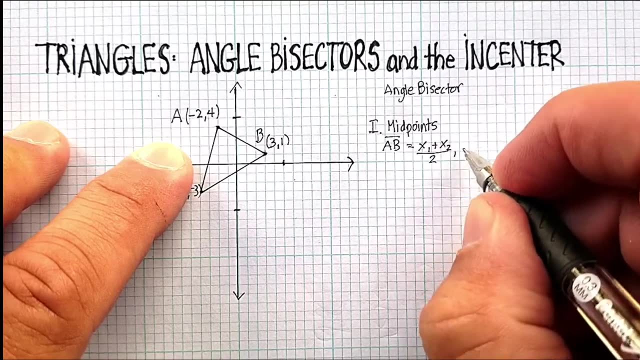 line segment A B, And A B goes from negative 2, 4 to 3, 1.. Remember that the midpoint formula is basically just add the x's and divide by 2, and you add the y's and divide by 2.. 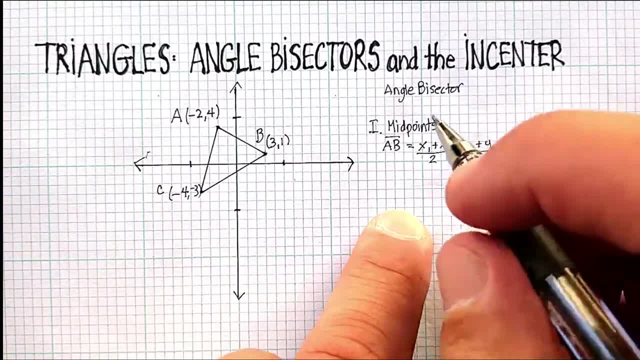 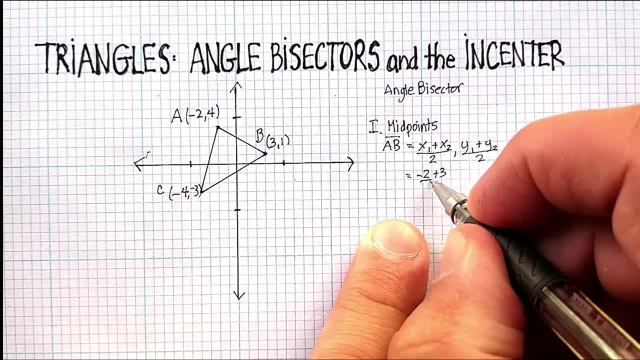 All right. So let's go ahead and just start plugging numbers in quickly. So negative 2 plus 3,. negative 2 plus 3, divided by 2. And for my y's I'm going to have 4 plus 1.. And again I'm going to divide by 2.. That's going to be negative 2 plus 3, divided by 2.. And for my y's I'm going to have 4 plus 1, and again I'm going to divide by 2.. 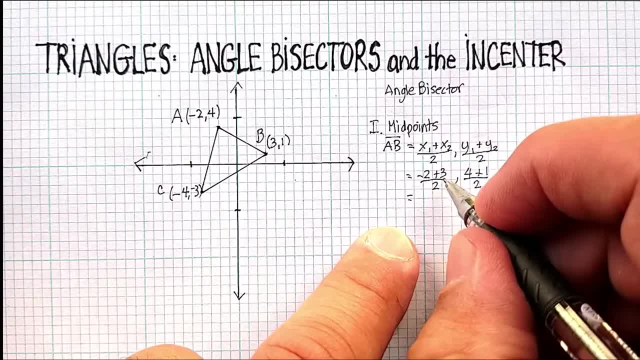 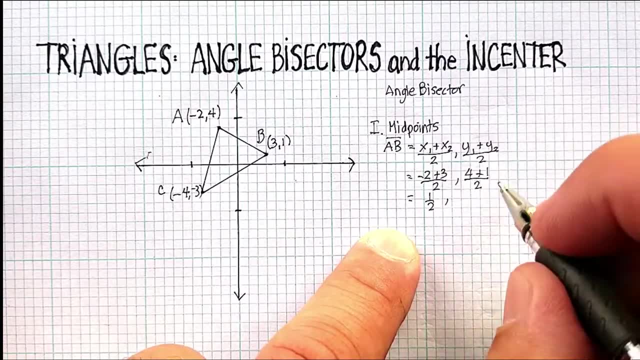 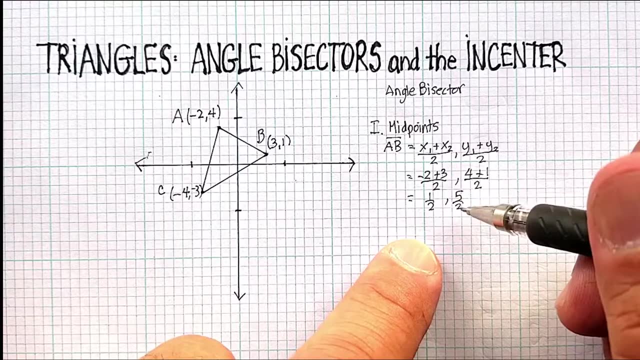 to give me negative. 2 plus 3 is positive 1, so 1 half and 5 over 2 is going to give me 5 over 2. if I want to change that to decimals, it would be 0.5 and 2.5. 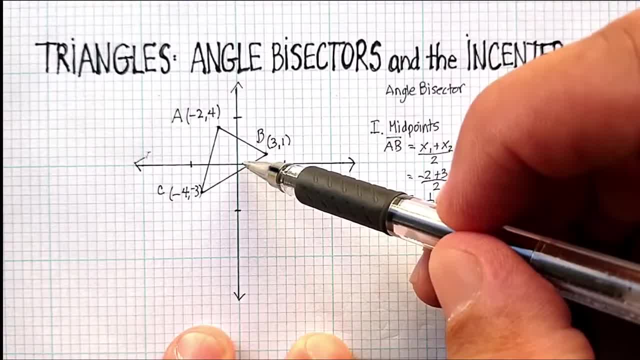 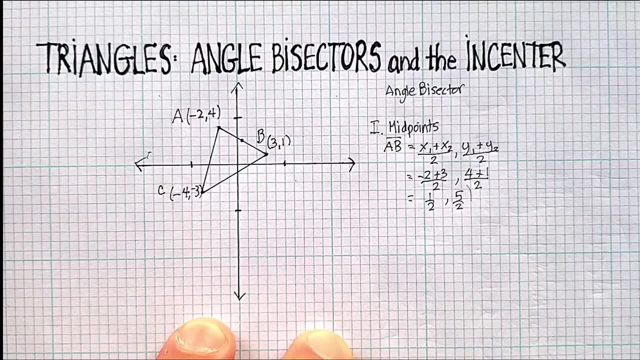 let's just check and make sure that's correct. so there's my half or 0.5, and then there's my two and a half. there's my midpoint, right there. let me just go ahead and mark that in a slightly different color. okay, so we have a little. 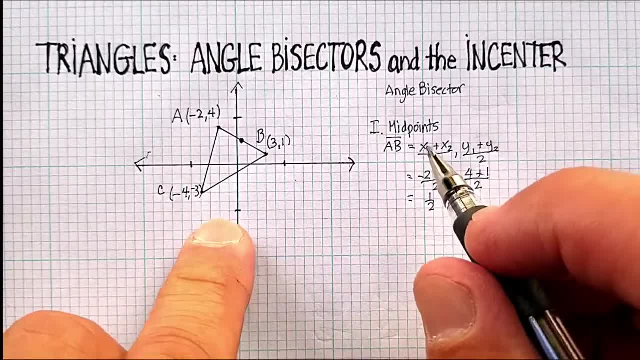 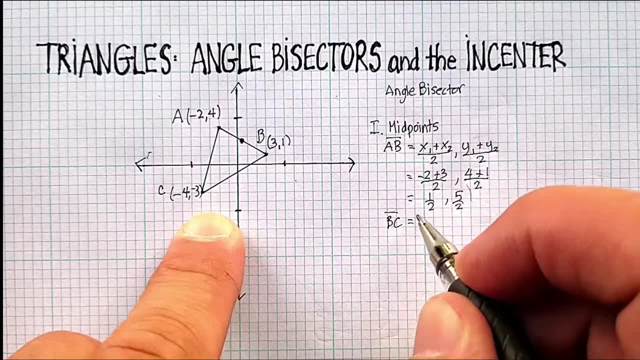 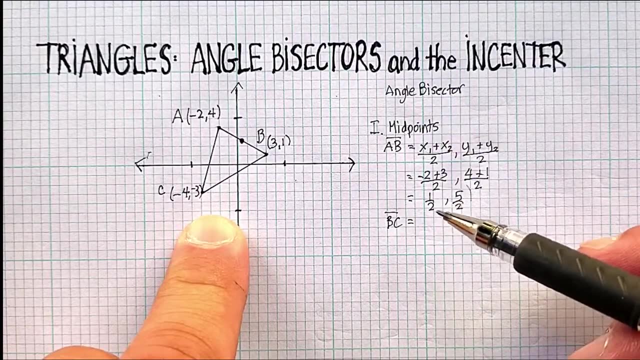 bit choice there. now let's try B C. let's find this site over here, B C. you know, in doing these problems, organization is really important, right? because you're essentially what you're doing is. you're writing to me a mathematical essay and you know each paragraph, if you want, of that essay. 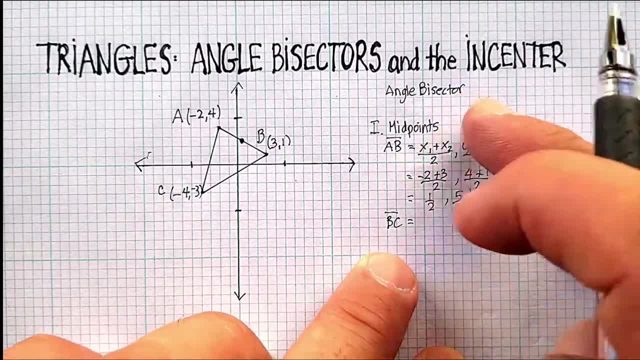 is in the middle, and if you're not doing that, then you're not doing that, because you're essentially. what you're doing is: you're writing to me a mathematical essay and you know each paragraph, if you want, of that essay is finding a very particular type of thing with calculations and text and headings. 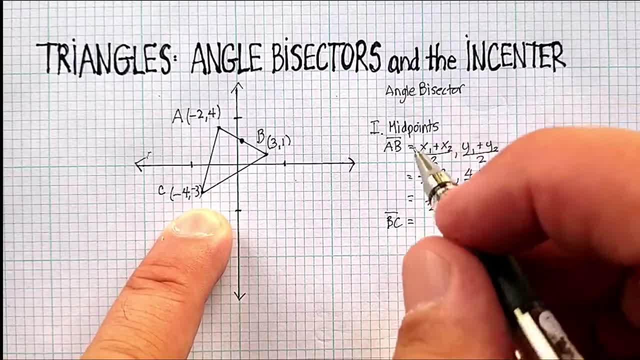 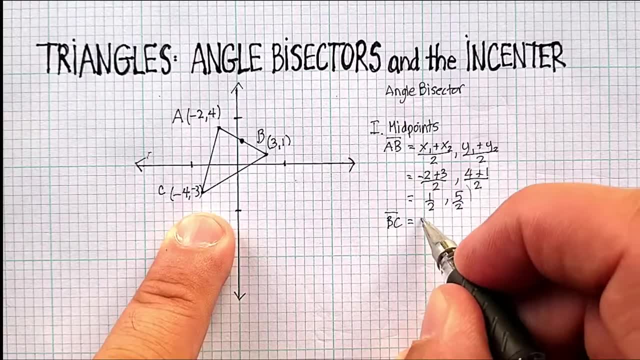 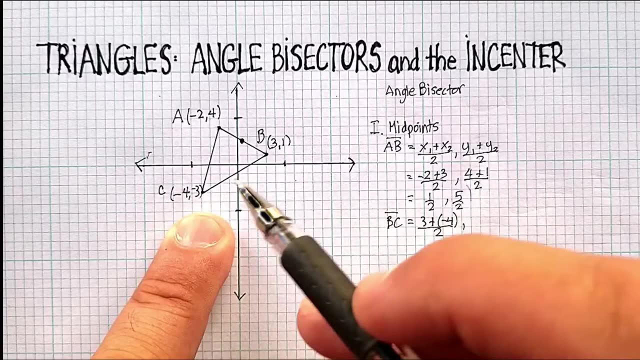 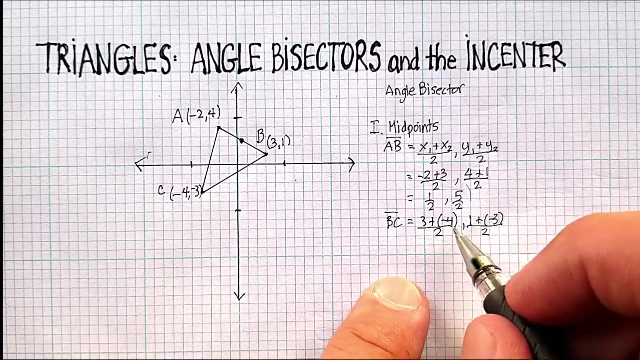 and that sort of thing. So try to keep it as organized as you can. So my x is 3 and my x2 is negative 4. So I'm going to say 3 plus a negative 4 and again divide it by 2, and then 1 plus a negative 3 and again divided by 2.. That's going to give. 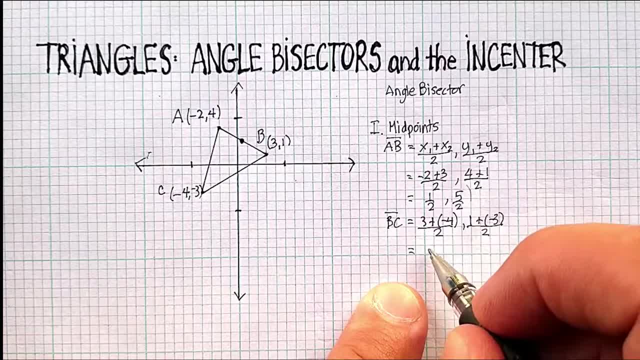 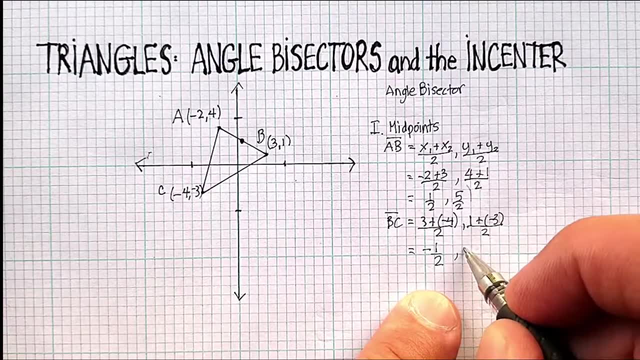 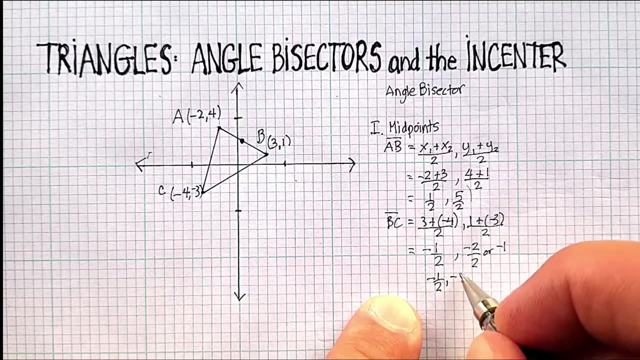 me a negative 1 over 2, which is a negative half, and that's going to give me what: negative: 2 over 2 or negative 1.. So negative half, negative 1.. Let's see if that actually makes some sense. So negative half, negative 1.. Sure enough it. 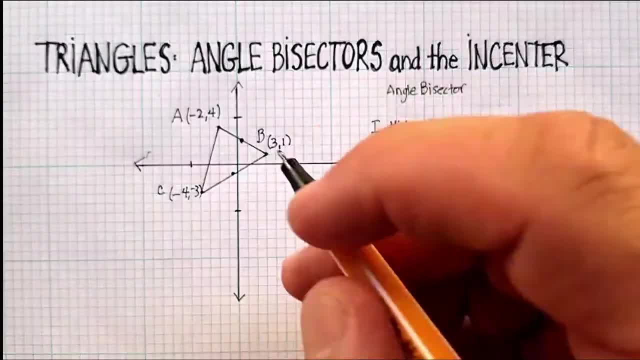 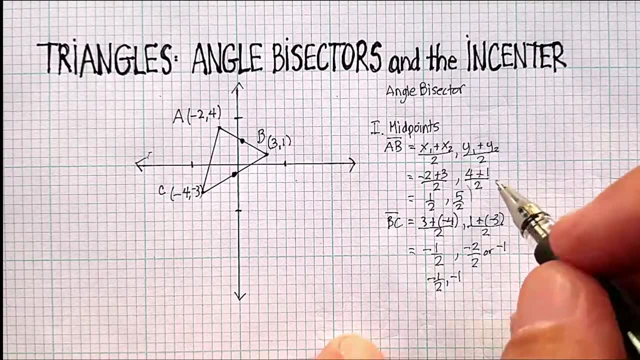 looks like it's right there on the line. Again, I'm going to mark it into this color here. I don't know if you can actually see the red, but it's actually a red. So I found my second midpoint. Let's go for a third. 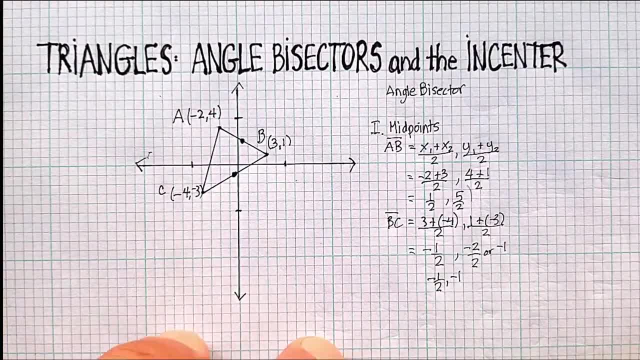 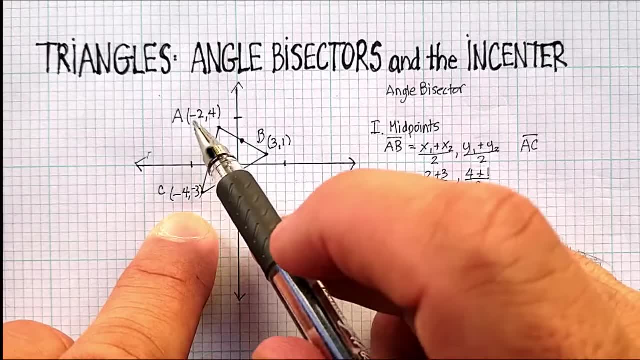 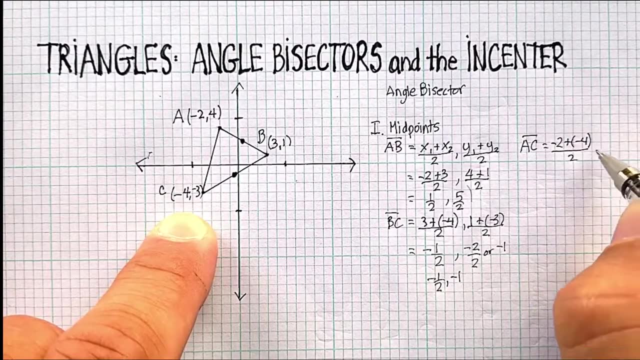 midpoint and that is a C. Okay, I'm going to put it up here. So line segment or side AC is negative 2, negative 4.. So negative 2 plus a negative 4 divided by 2, and then 4 plus a negative 3. 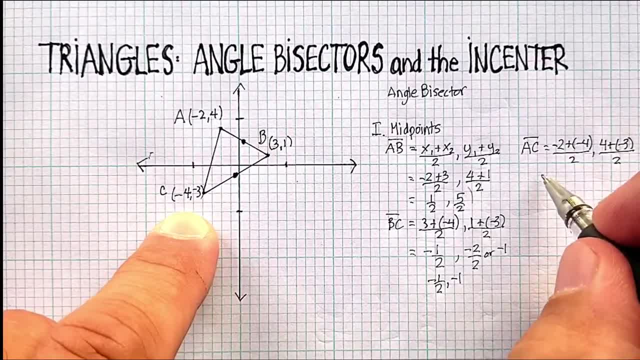 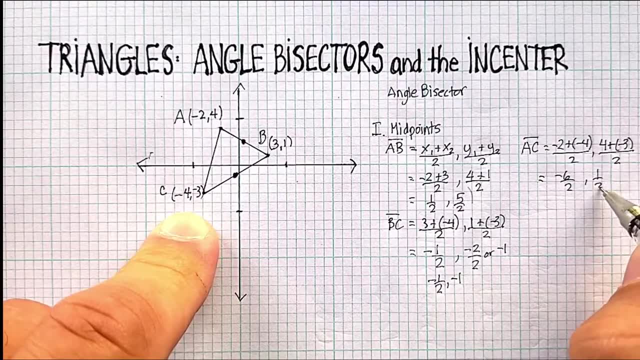 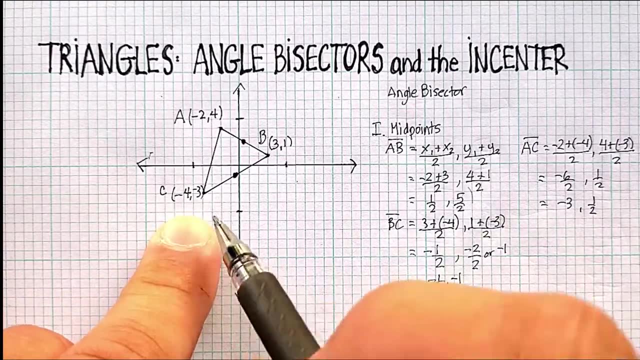 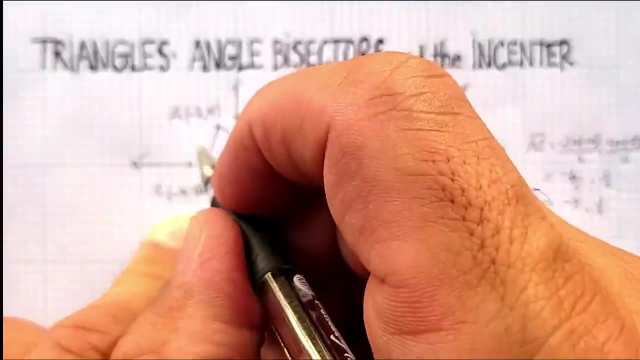 and again divided by 2.. That's going to give me negative 6 over 2, and that's going to give me 1 over 2.. Let's reduce this one and we get negative 3 and a positive half. Okay, so negative 3, sure enough, 1, 2, 3 and a positive half. right there and again it. 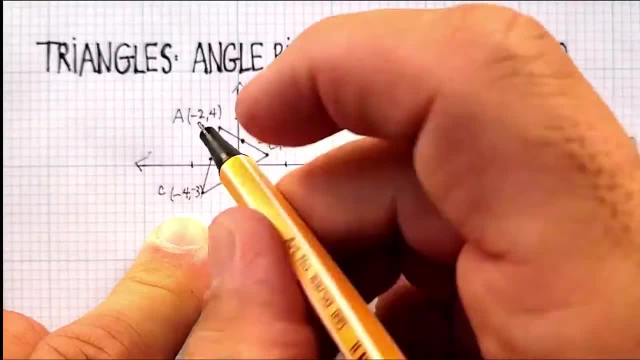 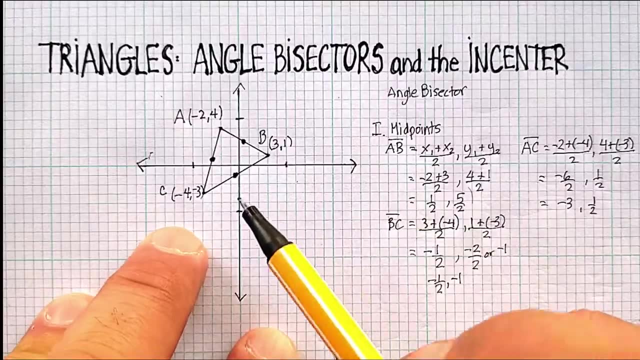 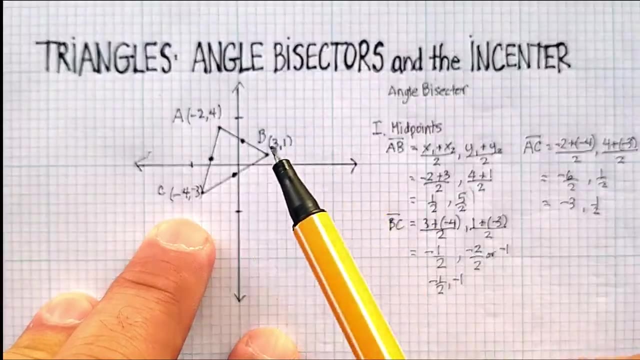 looks like it's dead on. So there's my other midpoint. So now what I'm going to do is I'm going to take a line and go from the middle of each of these vertices and I'm going to draw it to the midpoint of the opposite side. Now, 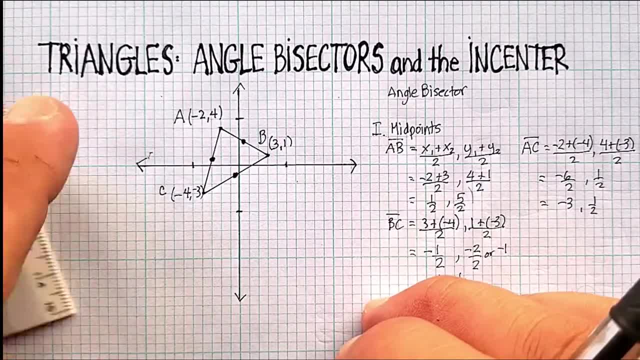 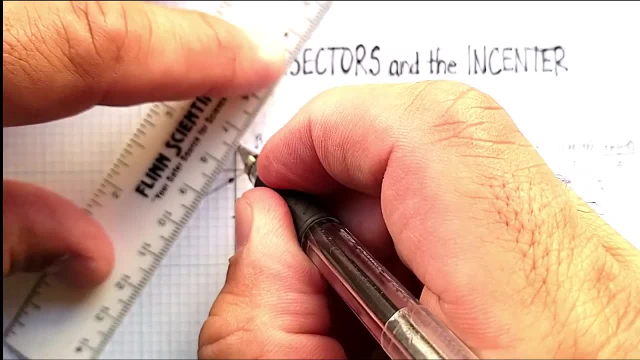 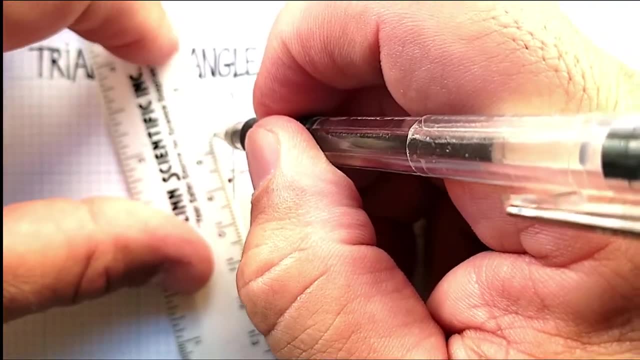 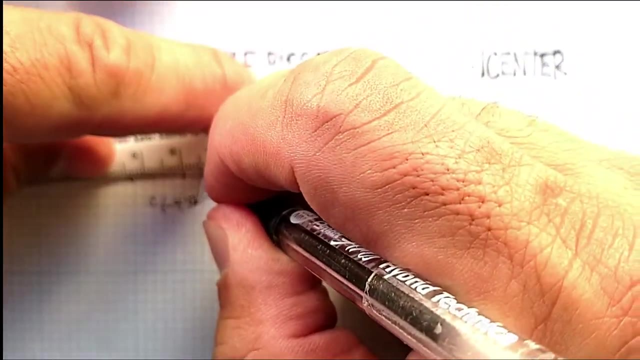 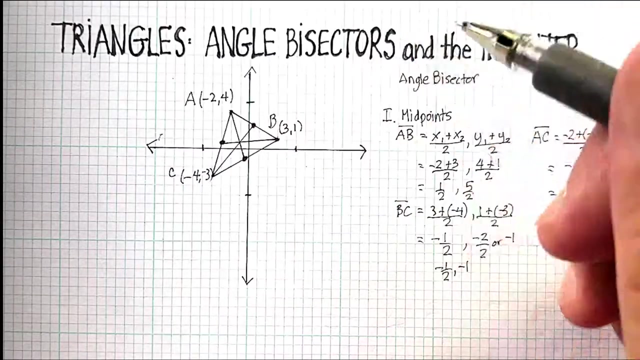 let's eyeball that first. Okay, I'm going to draw that by hand and I'll show you why here in just a second. So there's that one, There's this one and here's that one. Now I have an approximate of where my 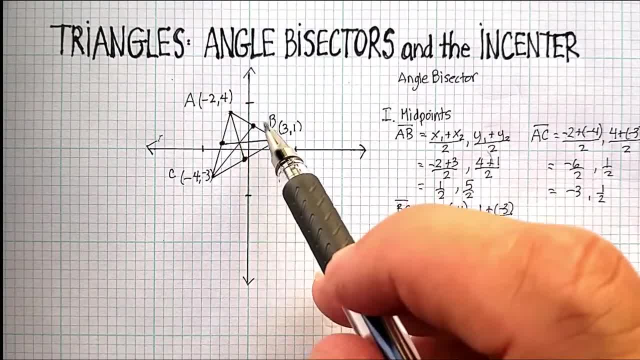 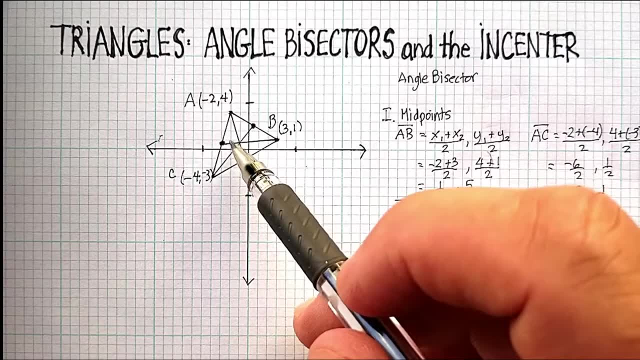 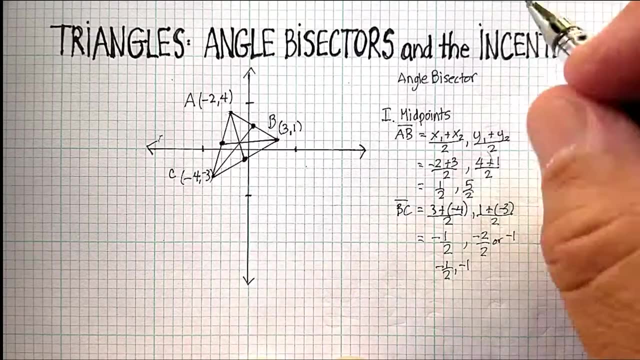 incenter is: and, again, the intersection of all three of those lines is called the incenter. Notice that it's not exactly on any one of the corners of my graph. So what do I have to do to find this mathematically? Because that's really what I'm doing here. 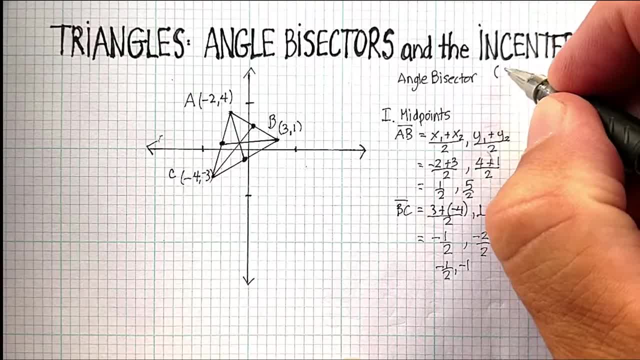 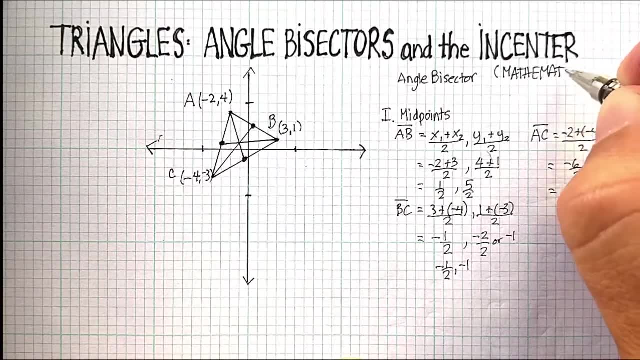 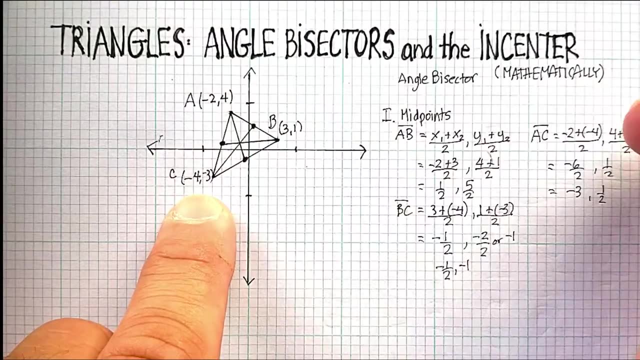 I'm finding this angle, bisector, I'm finding this in-center, mathematically. All right, That's important Mathematically, And I'm not just eyeballing it. How do I find out what this line is? Notice now, though, that I have two points. 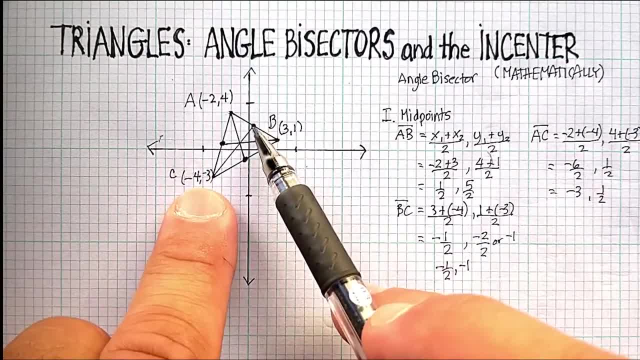 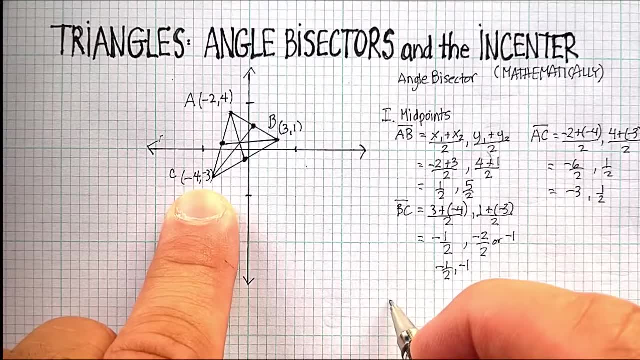 I've got this point, negative 4,, negative 3, and this midpoint, which I said was a half and five halves. So what I'm going to do is I'm going to take both of those points. Where do I have some room? 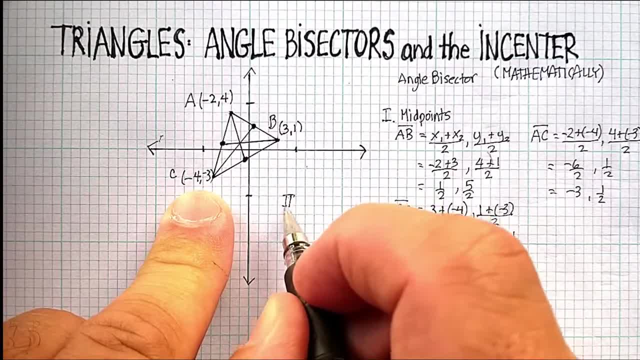 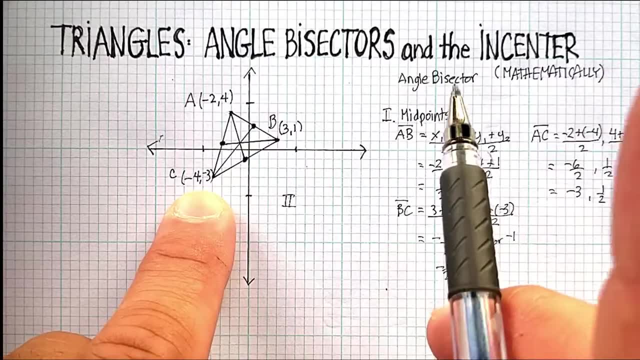 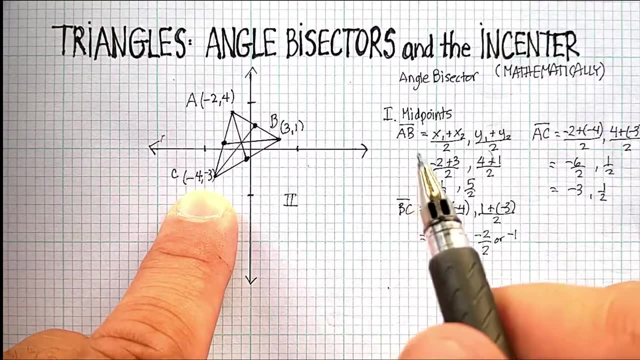 Here. Let's do it over here. So I'm going to call this second paragraph is finding the slope of the lines of the angle bisectors. Let me say that again, I'm finding the slope of the angle bisectors And if I didn't say it earlier, I think I did, but let me just make sure I've reiterated. 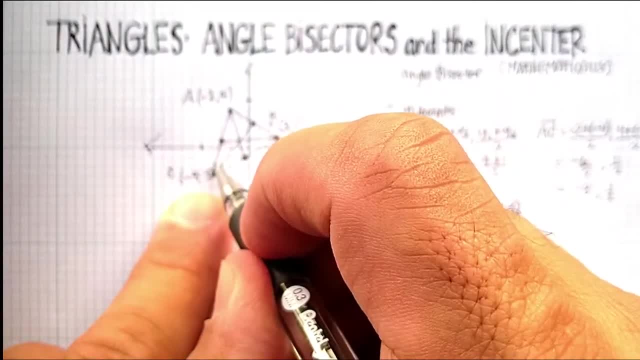 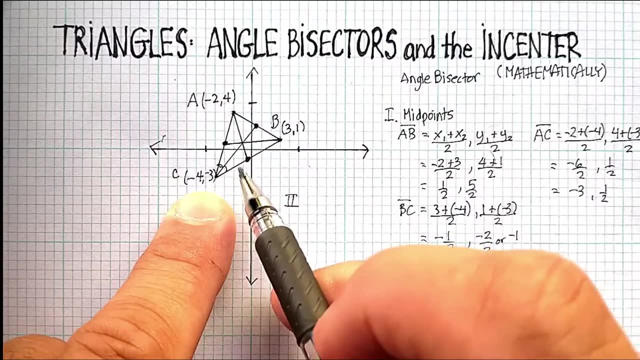 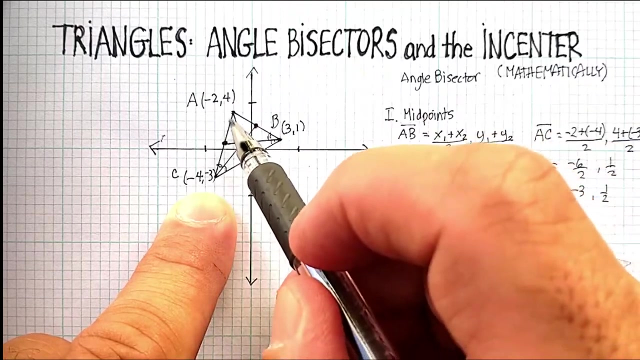 What I've done here is I've created angles. I've basically just bisected that angle and cut it in half. So this side, this half, is equal to that half Over here. this half is equal to this half. This half is equal to that half. 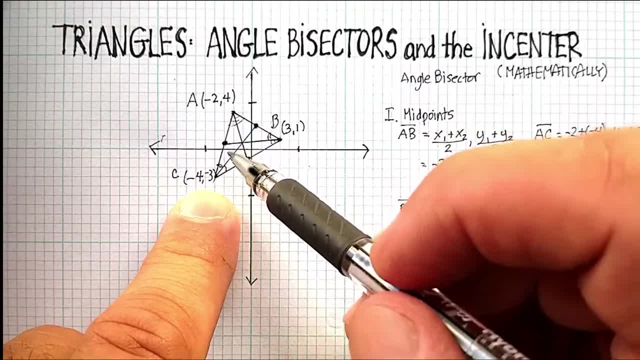 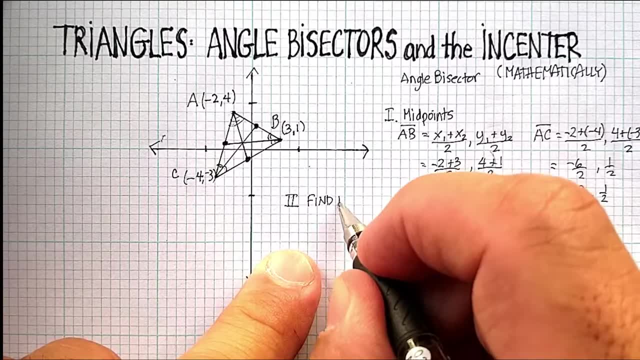 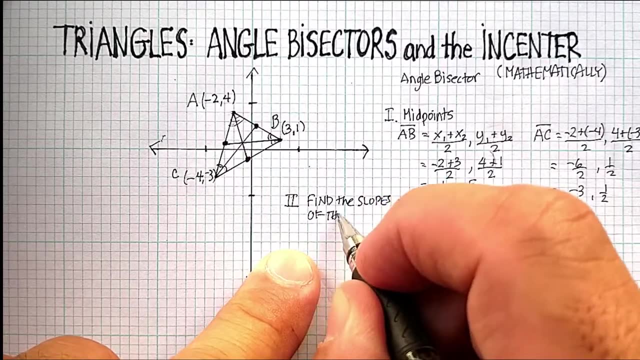 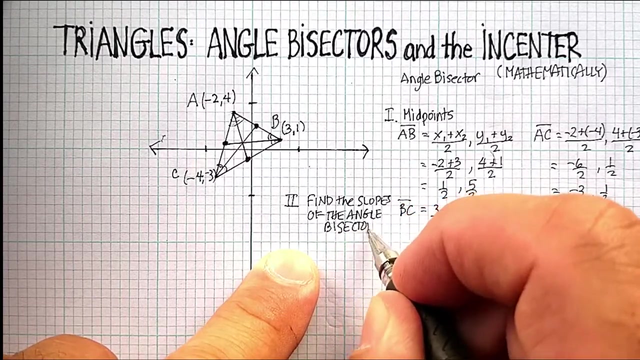 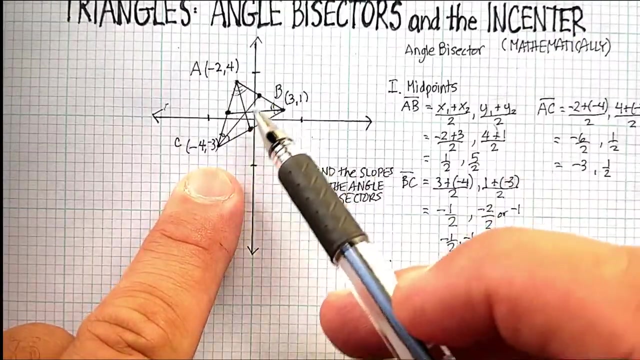 Okay, So that's important. You're cutting these angles. You're cutting these angles directly in half, So I'm going to find slopes of the angle bisectors, Okay, And again, you can do that because you have two points. Let's start with this one. 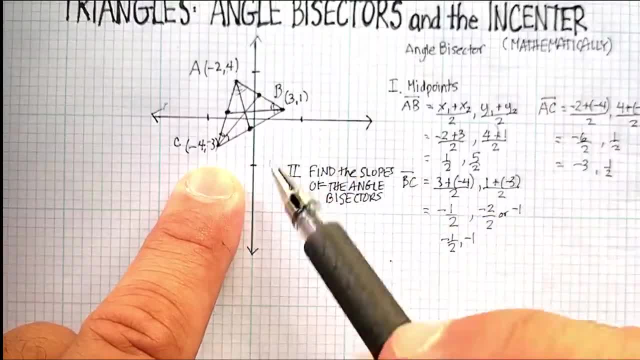 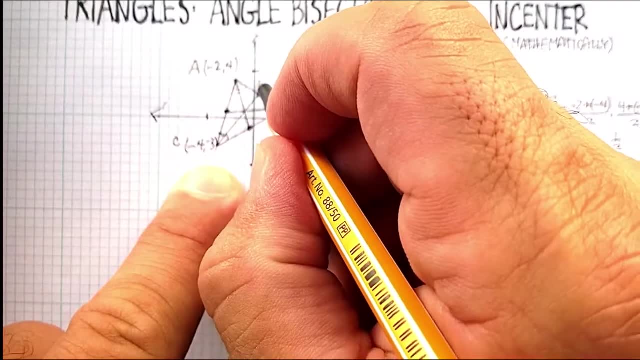 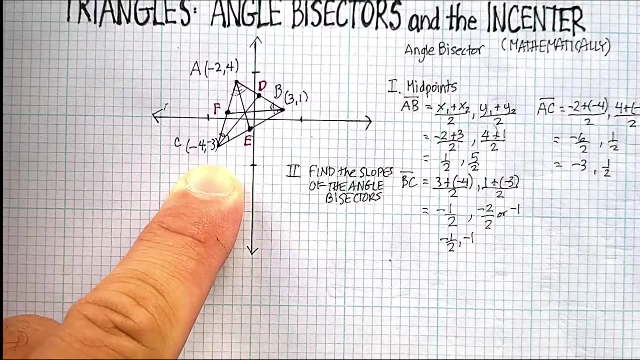 First, now, in order for me to do that, I probably need to give more letters here, right? So I'm going to call this C and I'm going to call this one here D, Let's go with D, Let's make this one E and let's make this one F. 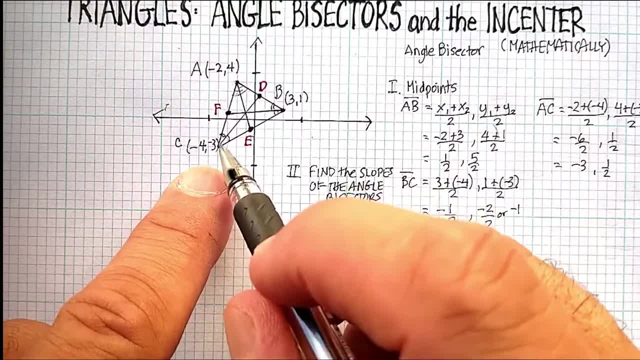 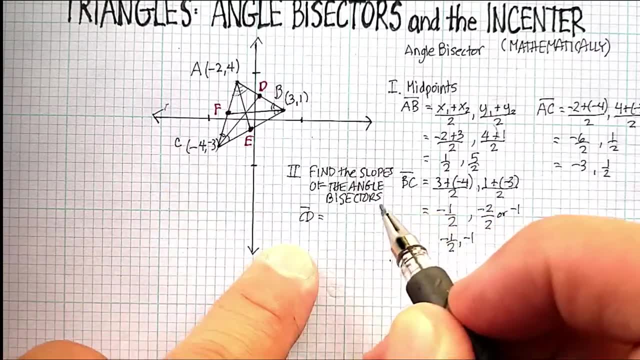 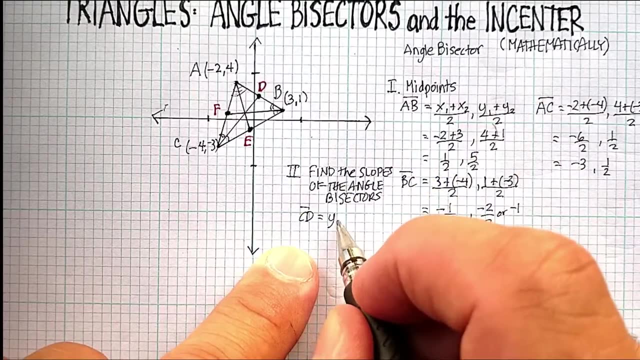 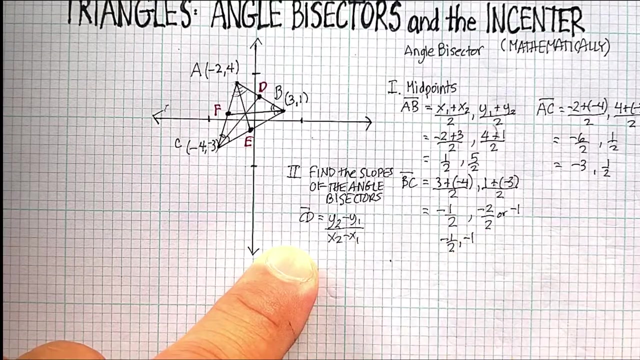 Okay, So let's find the line, the slope of line CD. All right, All right, And remember: the slope Slope is equal to the difference in the Y's divided by the difference in the X, Or slope is equal to Y sub 2 minus Y sub 1 over X sub 2 minus X sub 1.. 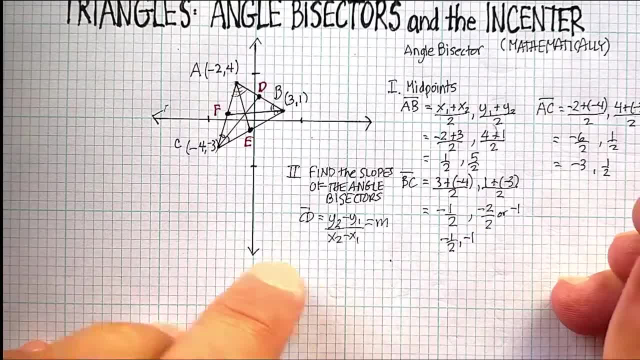 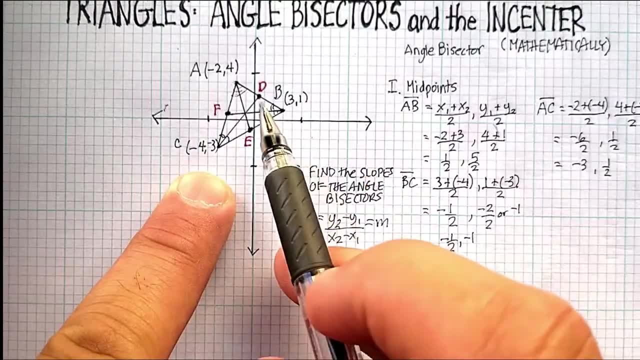 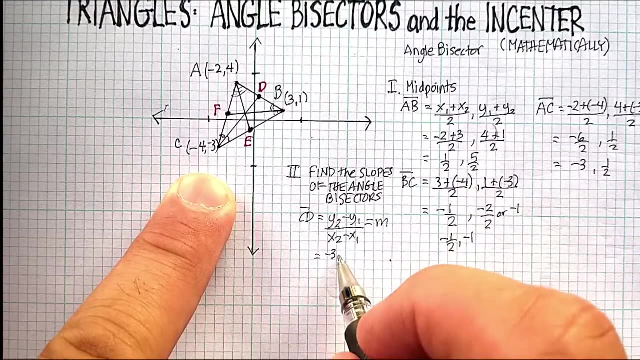 And remember that's equal to M the slope. Let's do the first one: Negative 3.. And we said that this midpoint here was 1 half and 5 over 2.. So minus 1.. Minus 5 over 2, which is just 2 and a half. 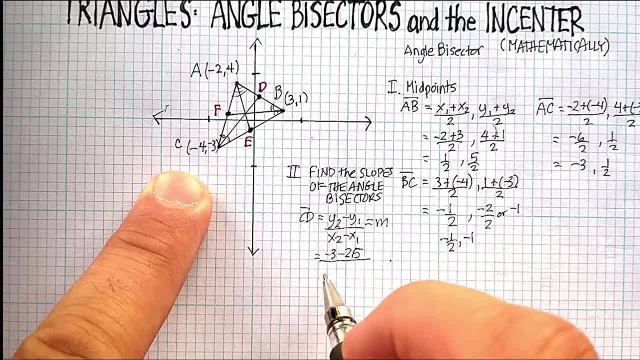 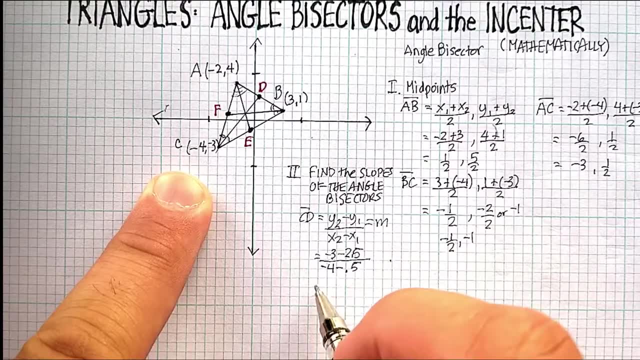 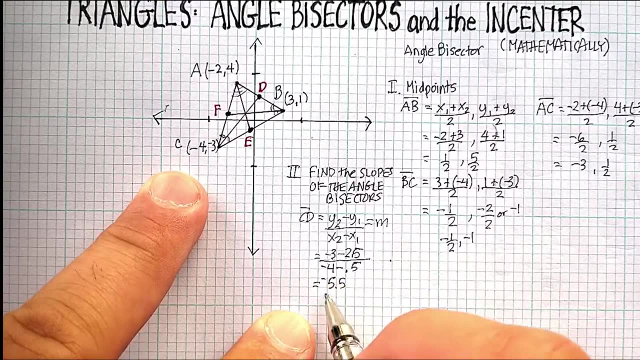 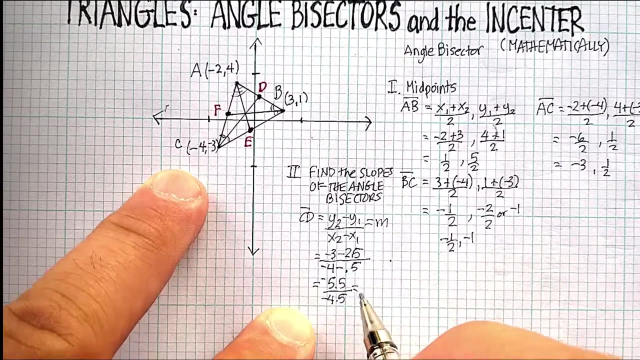 Over negative 4 minus half, which is just 0.5.. All right, Let's keep going. That's going to give me a negative 5.5.. And that's going to give me a negative 4.5.. Now, you should never leave a fraction as a decimal over a decimal. 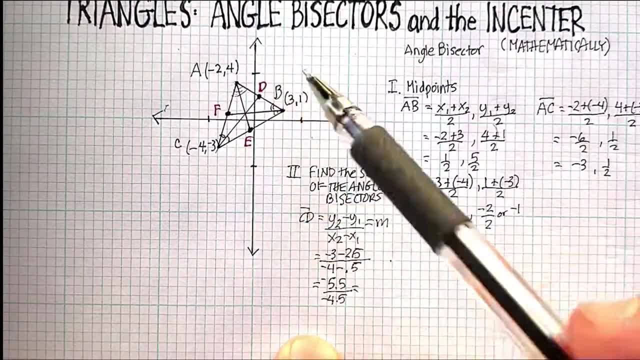 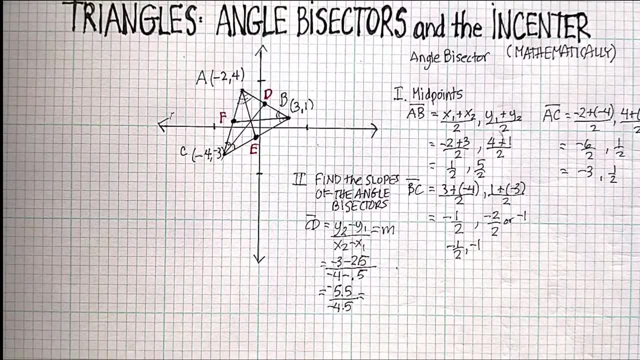 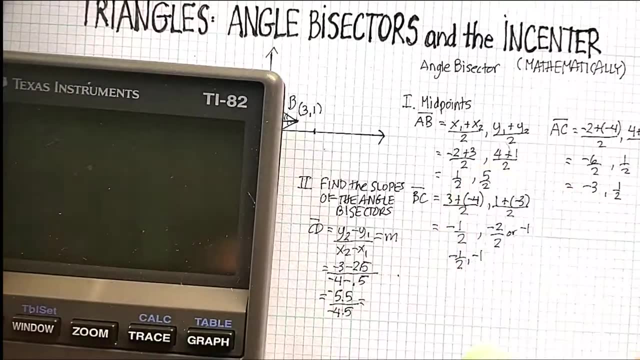 I do know that this is going to become a positive slope, and it makes sense because it's going up right, Because it's a negative divided by a negative. Let me just grab my calculator, And, And, So 5.5.. 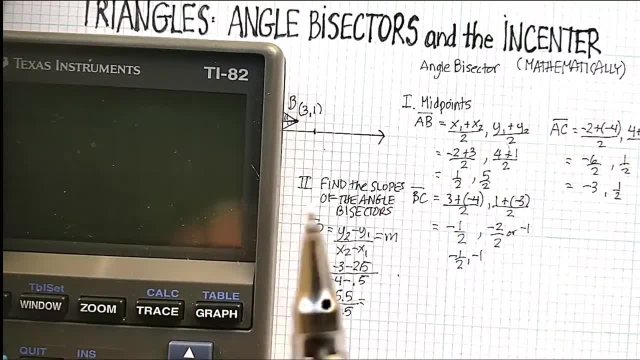 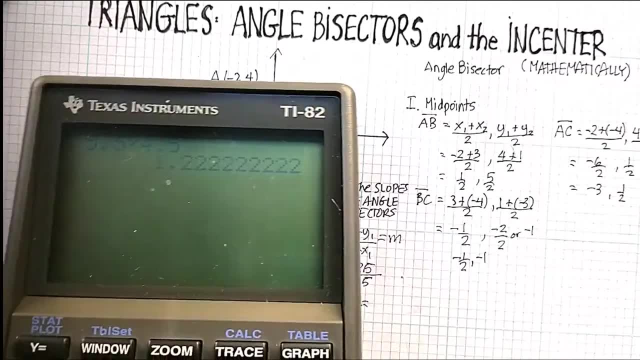 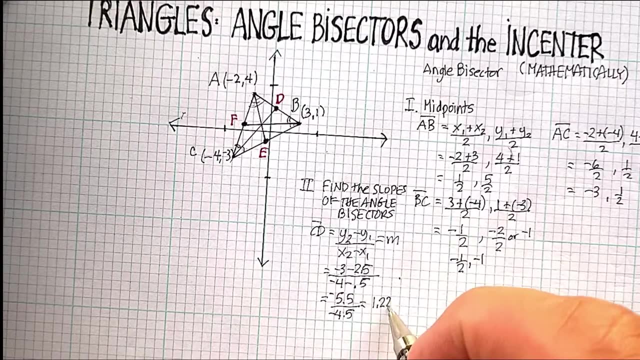 5.5.. Divided by 4.5, gives me a slope of 1.22.. I don't know if you can actually quite see that very well. 1.22 to repeating 1.22 is my slope. 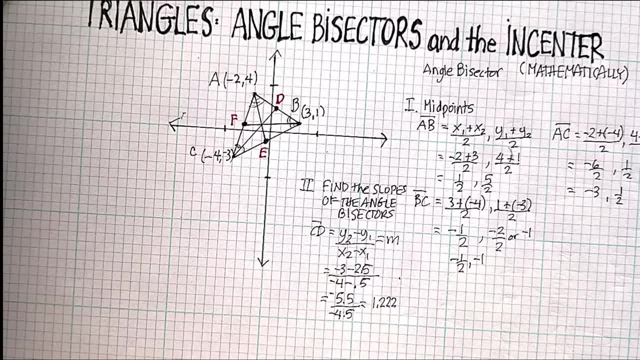 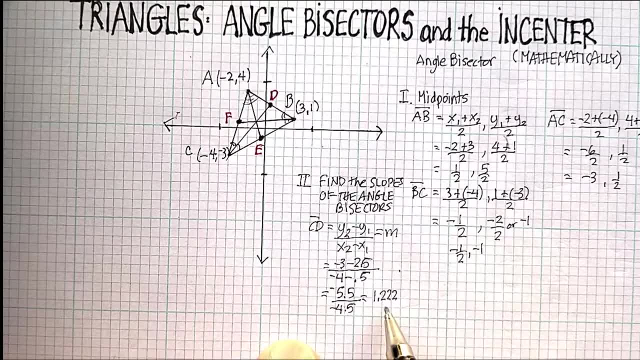 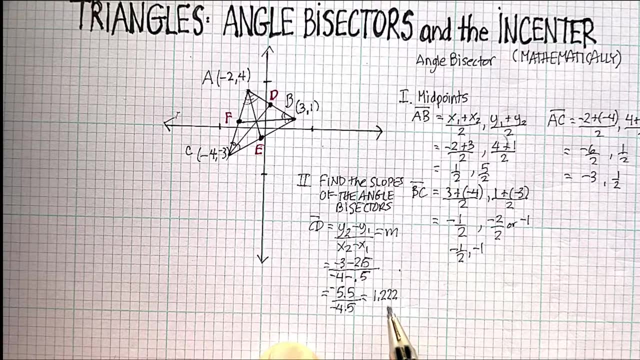 I'm toying with changing that to a fraction, But for right now I think I'm just going to leave it the way it is Okay. Once I have actually found that slope, I'm going to put one of these points and this slope into the point-slope form. 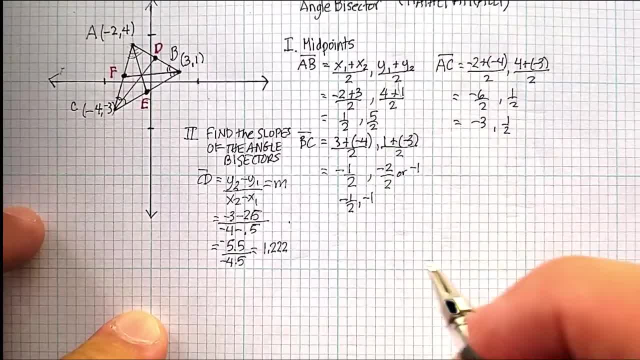 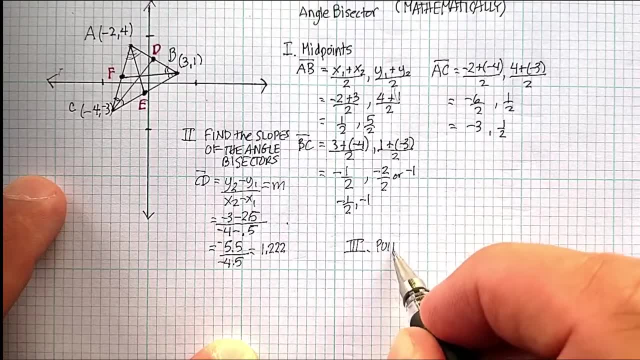 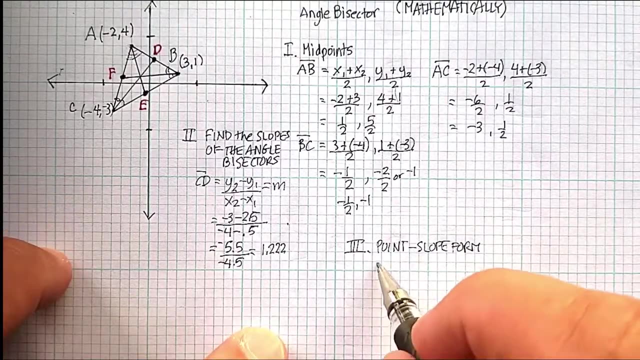 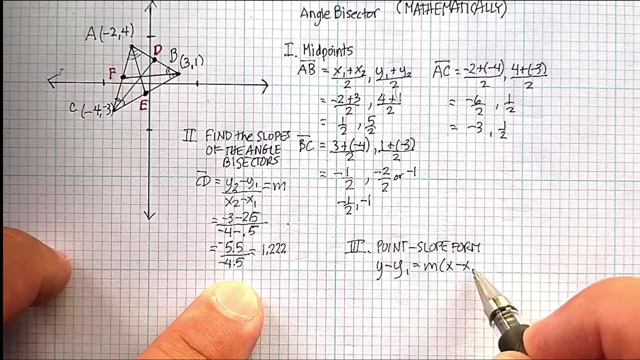 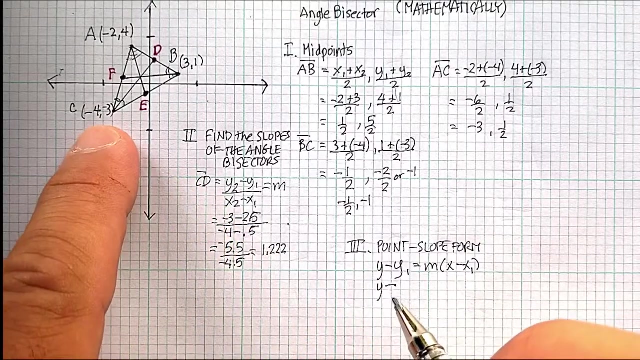 So let me make that my third paragraph. if you want Point-slope form, Remember, the point-slope form is y minus y sub 1 is equal to the slope times x minus x sub 1.. I'm going to put in y minus. choose either one of these two points. 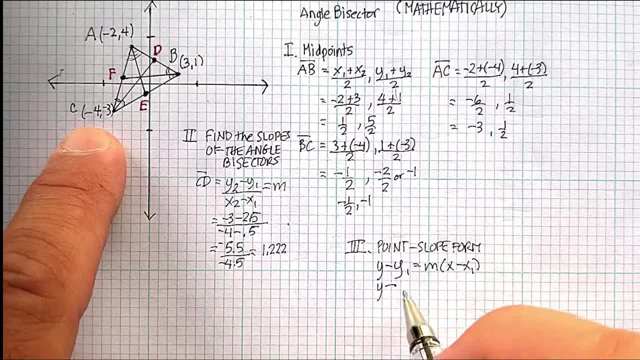 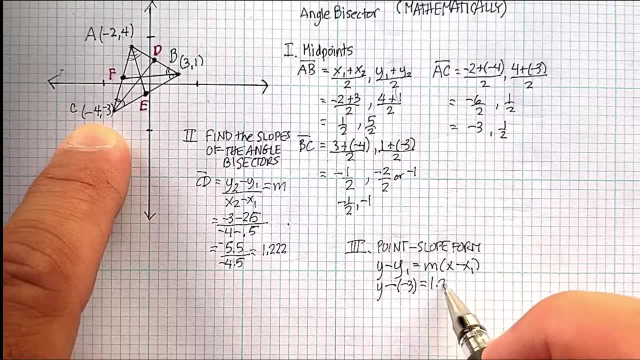 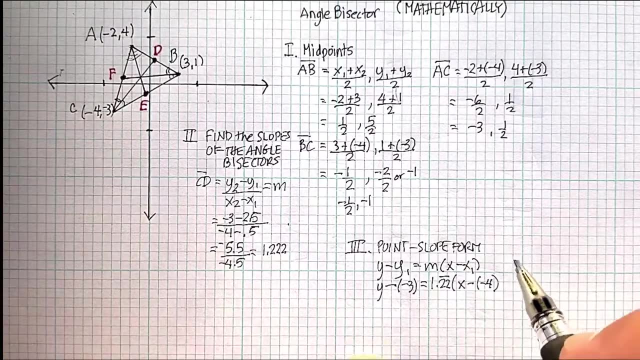 Let's just go with. let's go with the negative 4, 3.. So the y would be negative 3.. My slope is 1.22.. Let's just leave it like that. And then x minus a negative 4.. 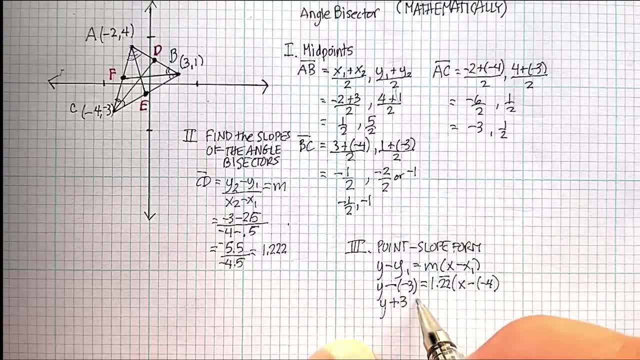 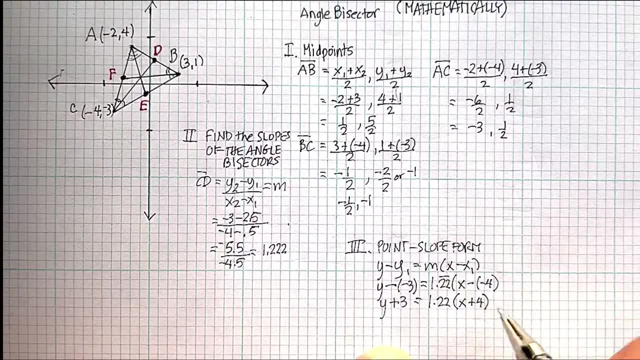 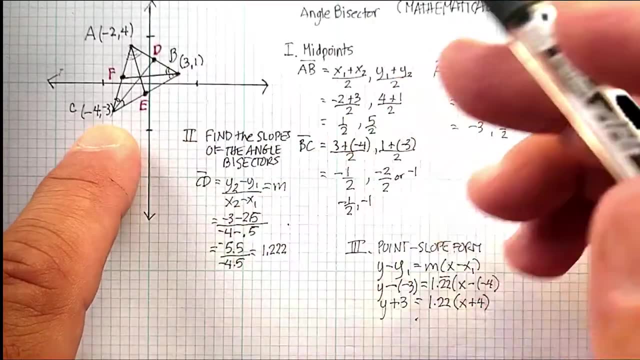 That's going to give me y And then x minus a negative 4.. Plus 3 is equal to 1.22 times x plus 4.. And that's the equation of this line. Okay, Now, what I'm going to do is I'm going to actually find the equation. 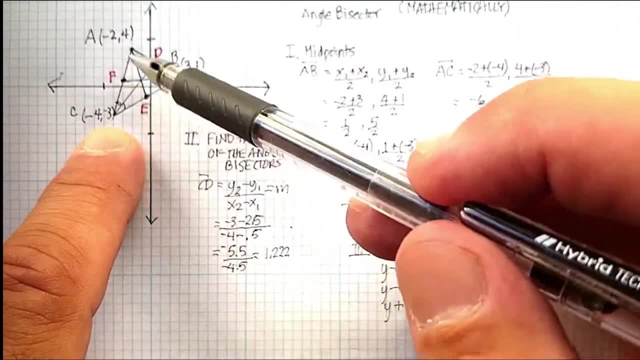 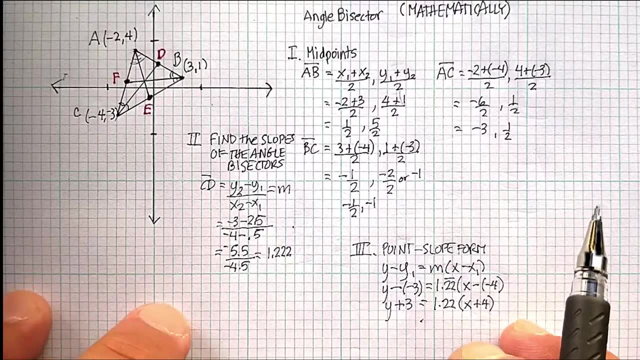 of each one of these lines, each one of these angle bisectors, And once you find the equation for each one of those lines, you can actually do- and this is my going to be my- step four. I'm not going to do the equation for each one just because it's going to take too long. 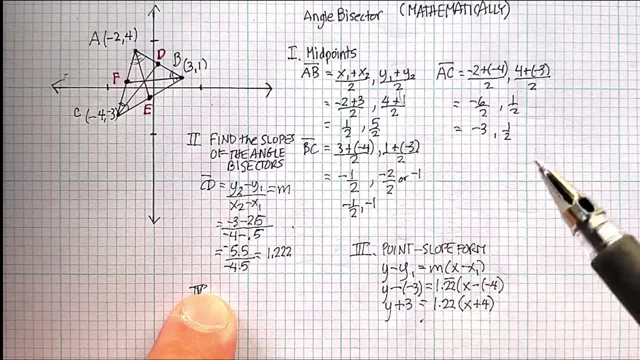 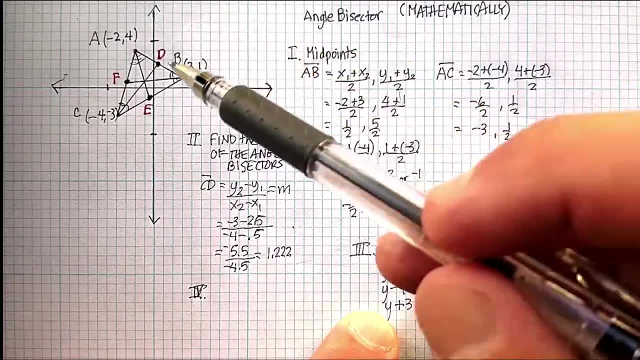 And this video is going to take a long, long time. You can do one of two things. You can put this into a graphing calculator. put all three of them into a graphing calculator and you should come up with a common point, right there? all right. 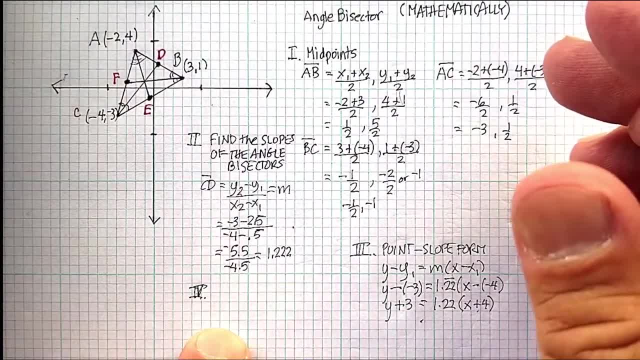 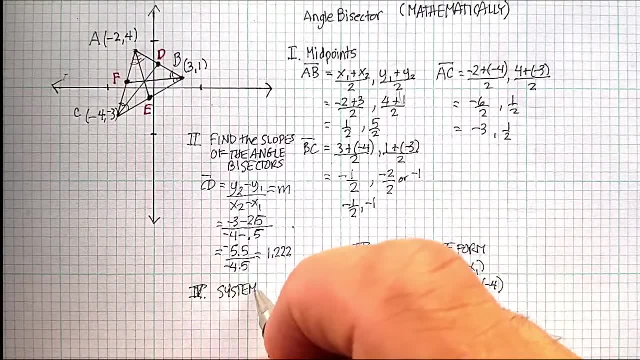 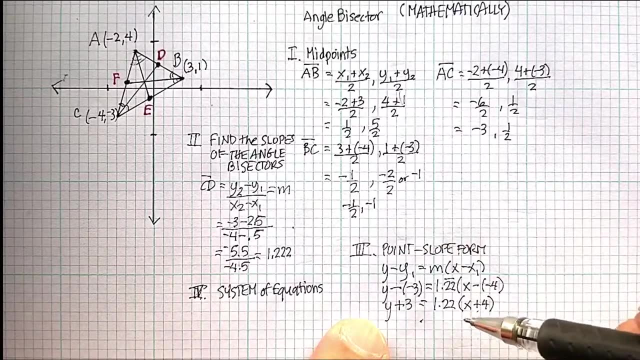 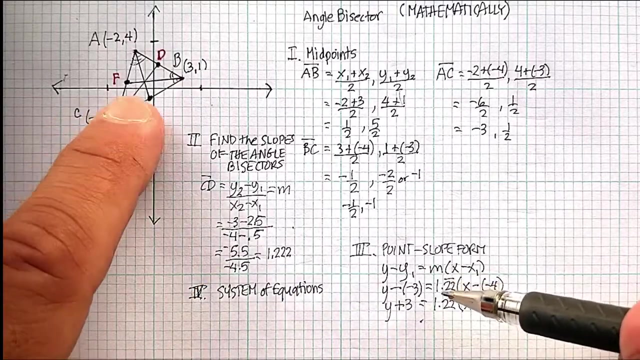 So that's step number one, or you could do step number one. The other thing you could do is just do a system of equations, Or you take all three of them and do a three by three system of equations, right? And then you could find out what the common point is for all three. 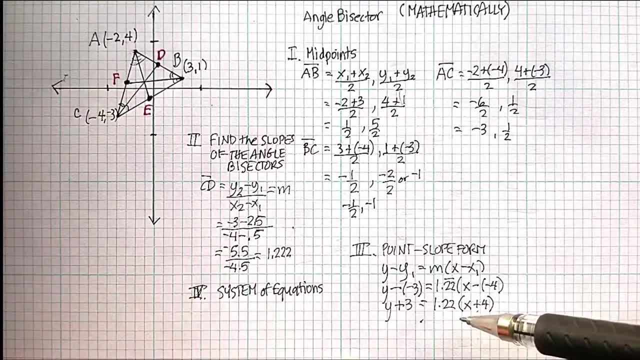 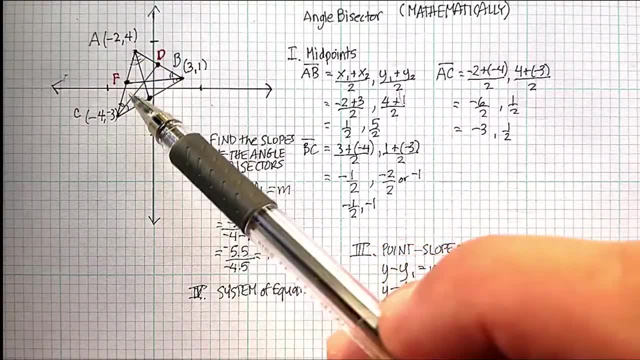 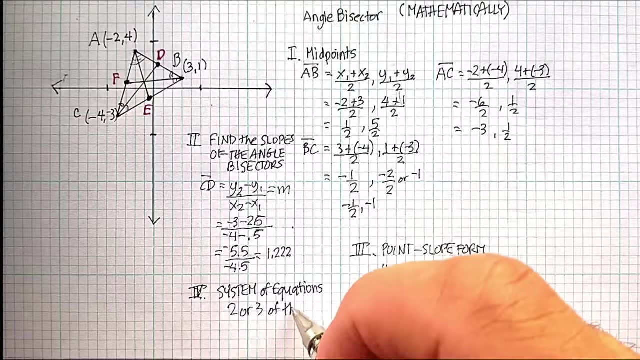 Or you could just take two of them and find out a two by two system of equations And then, whatever that common point is, you realize that it's going to be the same for all three of them. okay, a system of equations for two or three of the lines. And again, I'm not going to do. 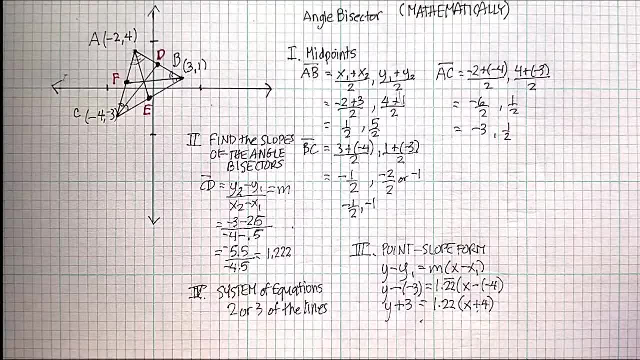 that, because it's just going to take too long for this very long video. Okay, I hope that was helpful to you. 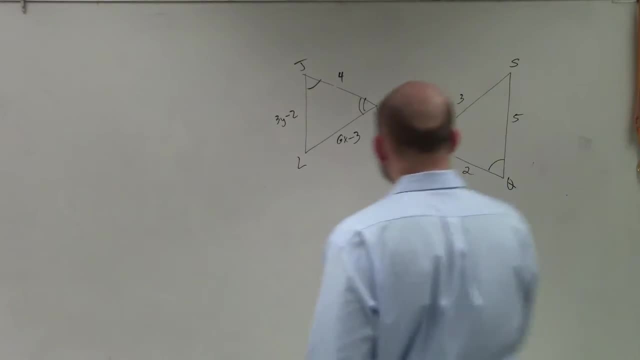 OK. So in this case, ladies and gentlemen, what we have is we have two figures And I believe it does say JML. So actually, they do already tell us triangle JML is similar to triangle QFS. So this is something they tell us in the problem. 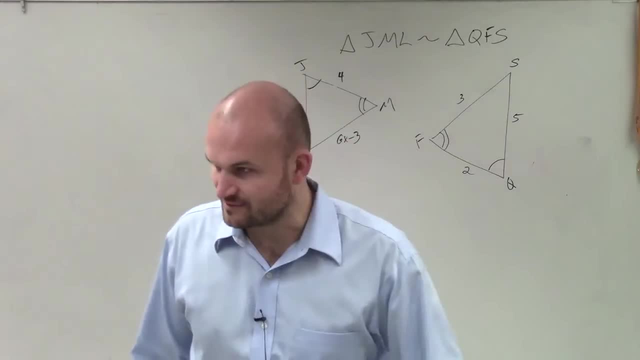 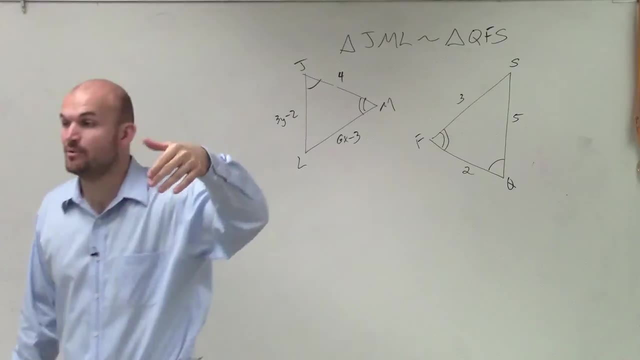 So you're provided a problem, Carly, And here's the information you're given. You're given these two figures and they say they're similar to each other. That means they're proportionally similar, but they don't necessarily have the same size. 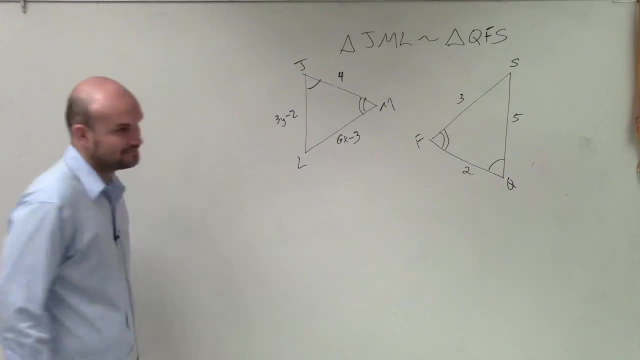 And they want us to solve for x and for y. Now we can write a. what I would like to do is go ahead and write in some proportions. We know that the angles- obviously you guys can see that Q and J are congruent, right?